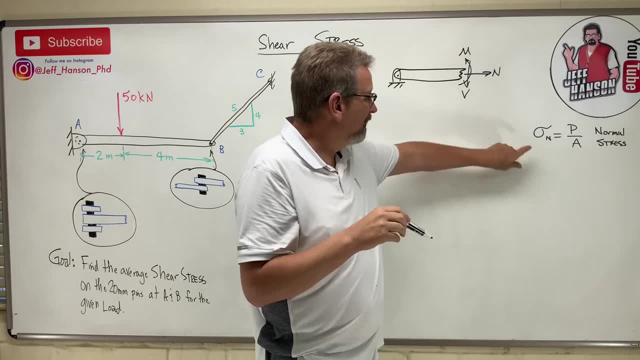 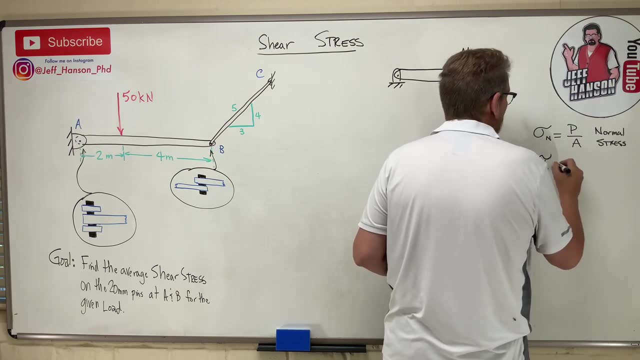 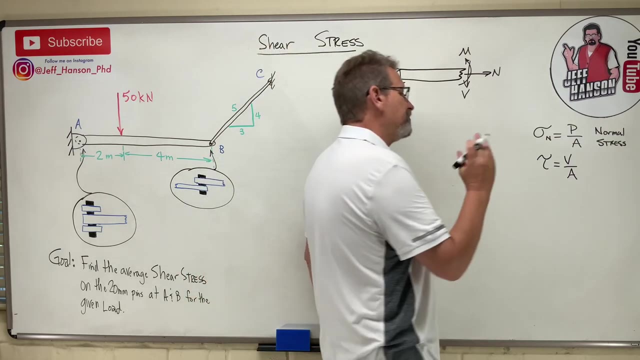 going like that, right, What's the intensity of the force? So guess what? we get on our equation sheet over here, A new equation for the day, and that equation goes like this: okay, Tau equals, and let me, I'm just going to change this. okay, I'm going to put just so. 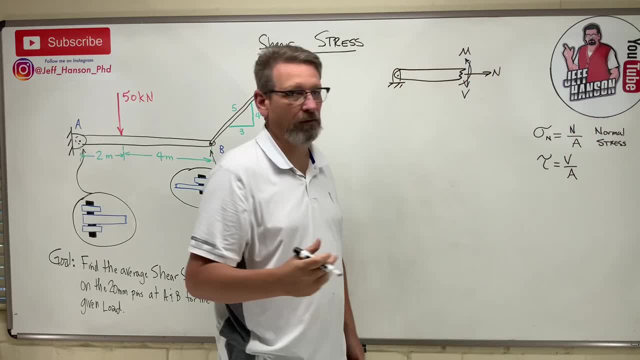 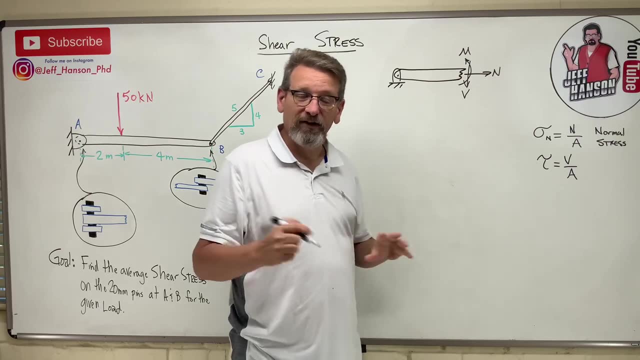 we're clear on that. I'm going to put an N there for normal right, Because it's that one that does normal stress and it's V that contributes to sheer stress, okay. So that's that force that's tearing it in half in that direction, okay. 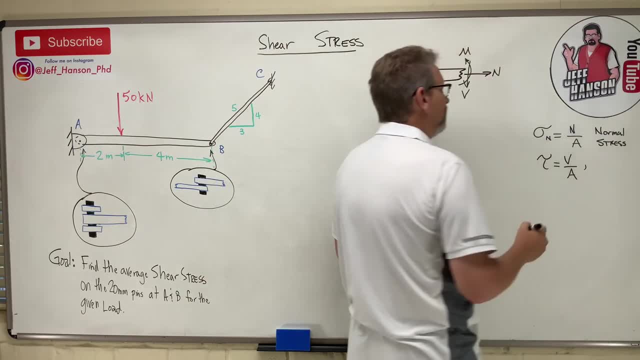 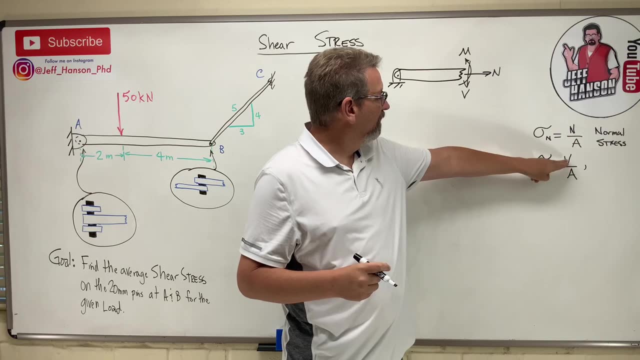 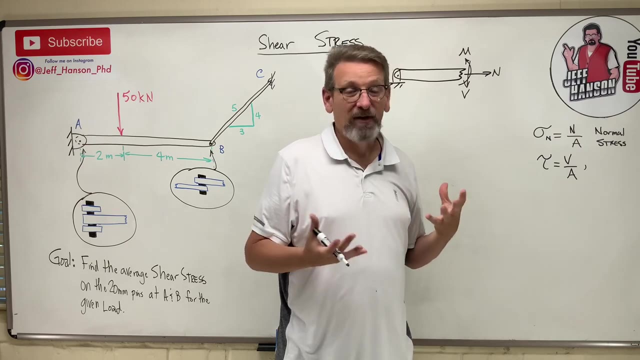 Now that we have one more additional equation, and this equation, this is the Greek letter tau, for sheer stress. the equation goes exactly the same as it did up here: V is just a force, and so A is area, and so the units are exactly the same, but it's a different kind of stress. 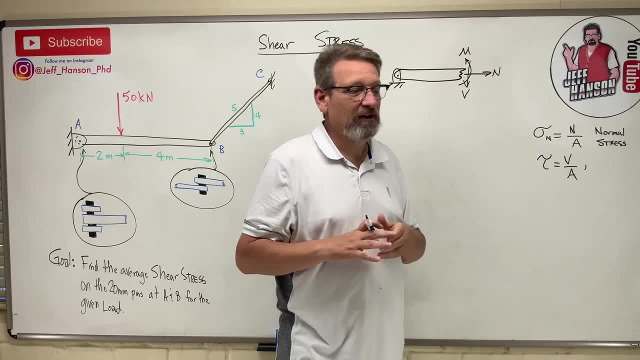 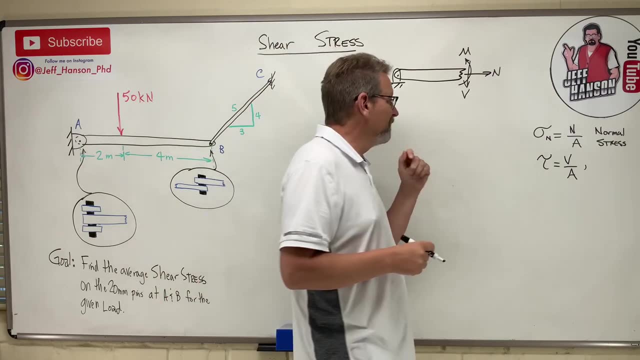 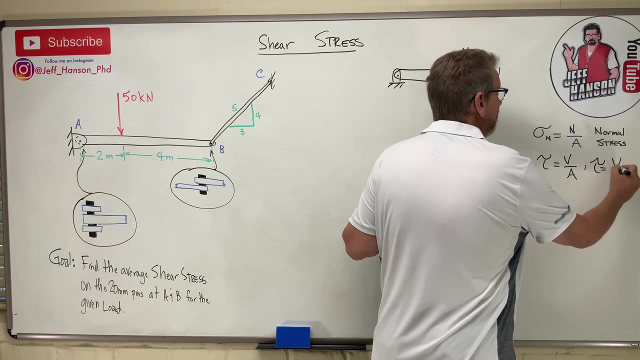 than normal stress. So you got- you can't get those two confused. and the way I think about sheer stress is just a tearing stress, just it's trying to tear something in half. okay, And let's see what else do I have over here? Oh yeah, how about this one? Tau equals V over. 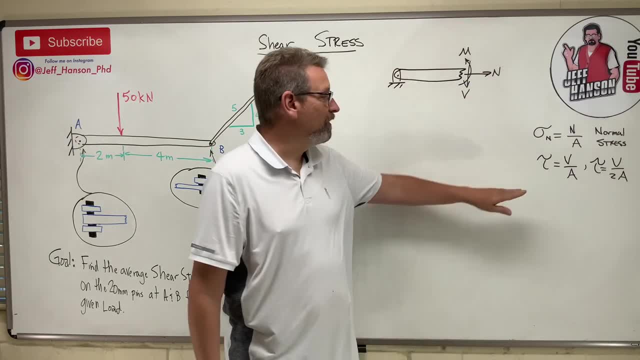 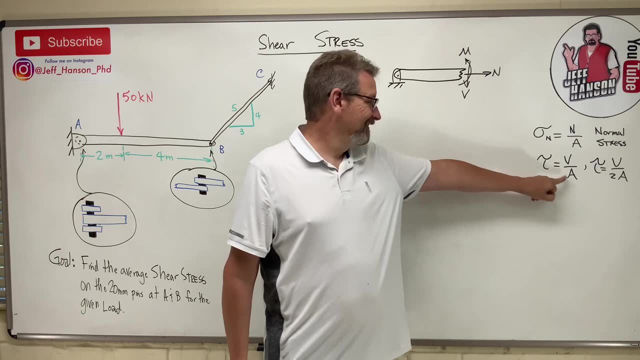 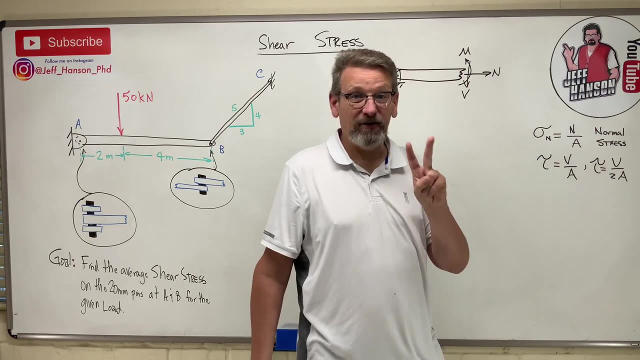 2A. okay. So what you can have here is you can have shingle single sheer- say that three times fast- or you can have double sheer. The 2A is for two areas, because you're having to sheer through twice as much area as you do for a single sheer. 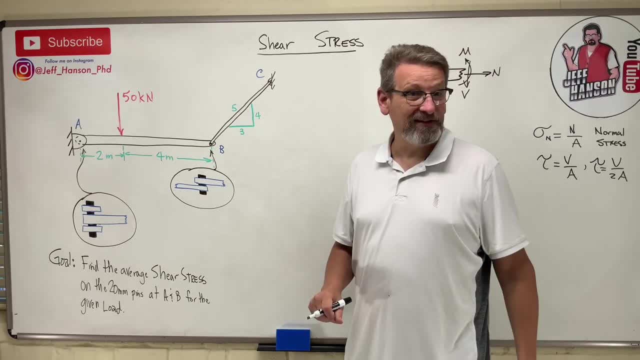 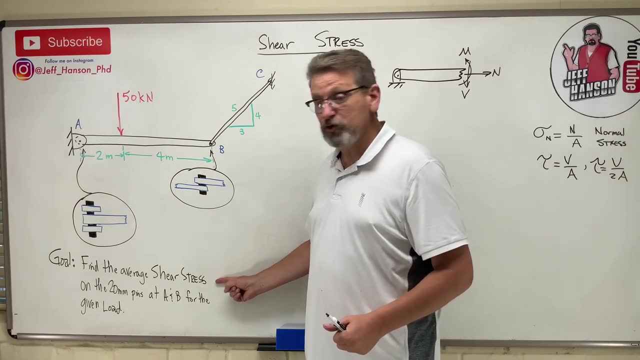 Let's look at a problem, bam, and let's see if we can see that. okay, Now, where we see the sheer that we're looking at here. this one says: find the sheer stress on the 20 millimeter pins at A and B. So we have a pin connection here and a pin connection there. 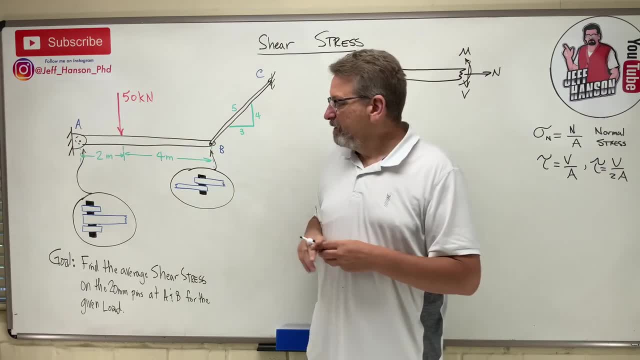 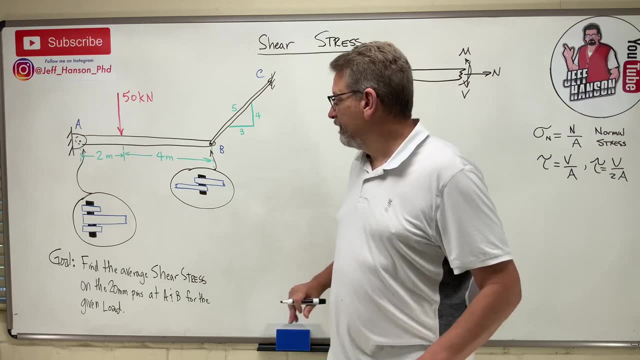 Now, in statics, a pin connection was a pin connection. who cares? right. But in solids, when you say you got a pin connection you want to like, okay, what kind of pin connection? Is it a single or is it a double? sheer, right, And here's some pictures. right, Here's some. 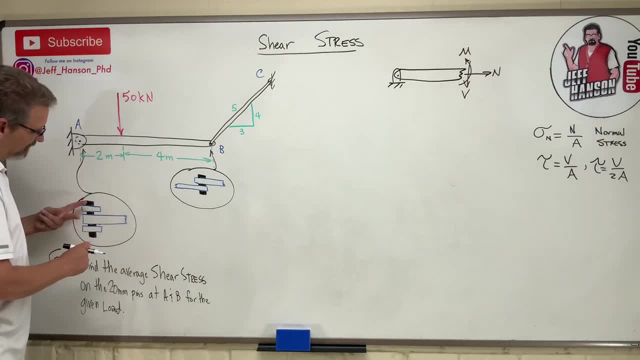 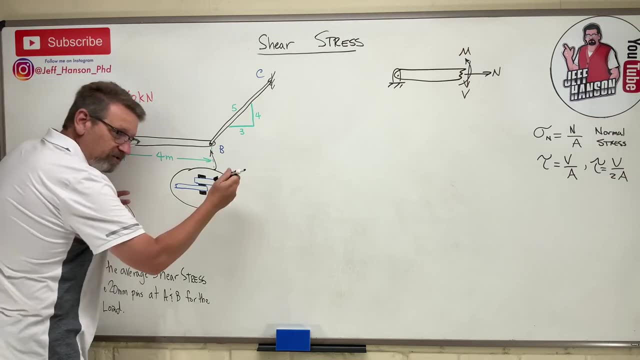 explicit pictures of a single sheer right. And here's some pictures right. Here's some loaded views of that pin. So here you can see there's two, and then the beam is in the center. there The pin goes through the whole thing. So in order to tear that loose, what do you have to do? 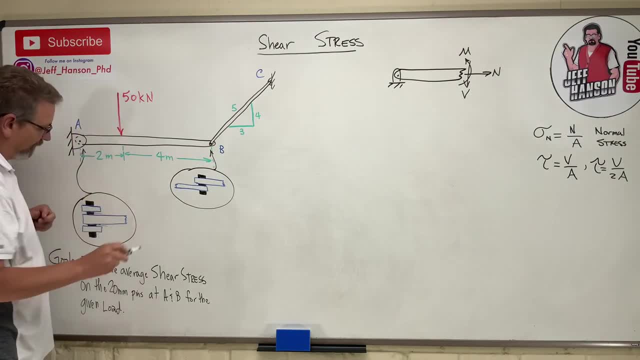 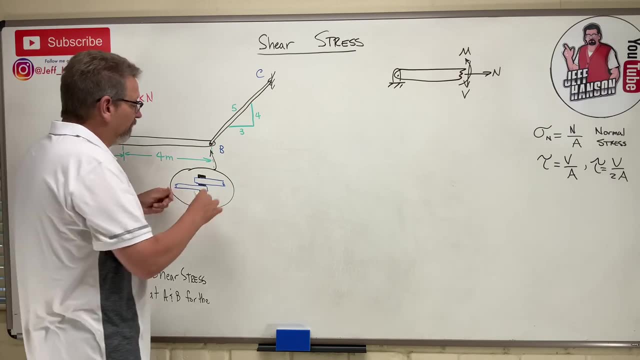 You would have to tear through here and through there, right? So that's what a double sheer pin would look like. okay, This one over here, right? If I pull on this one that way, right, And pull on this one this way, then I have to sheer that pin. But how many times do I have to pull on this one? 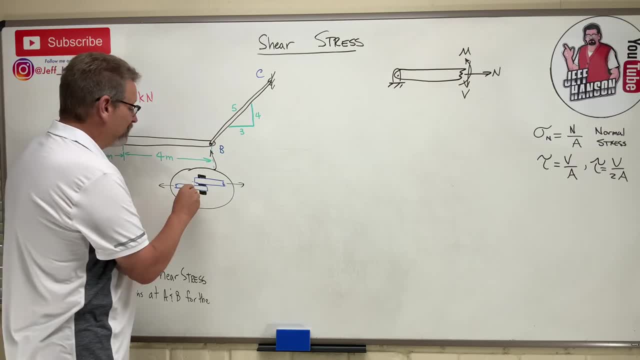 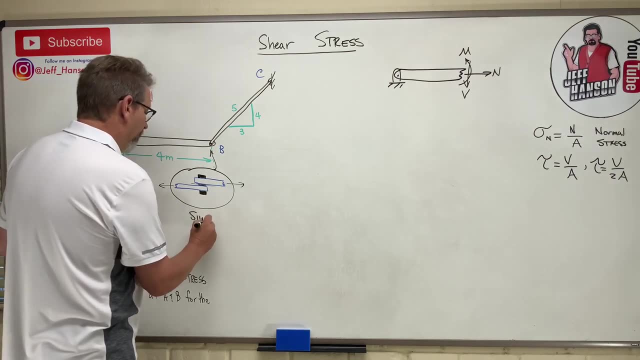 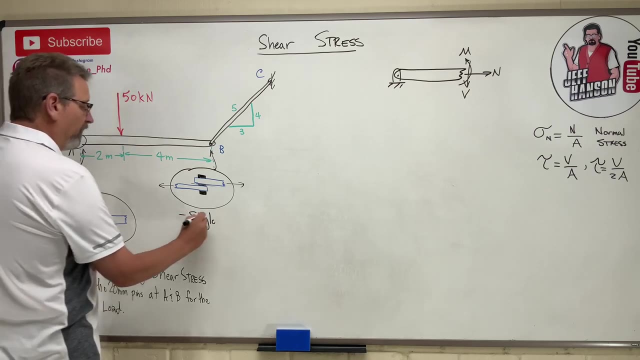 How many times do I have to sheer that pin to make it fail? I only have to make it sheer- whoop right through there one time to make it fail. That is single sheer. So this is single and this is double. okay, And all these problems, they'll have a little blow up of the pin. They. 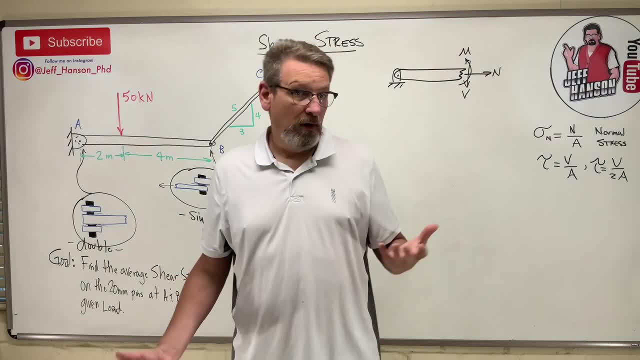 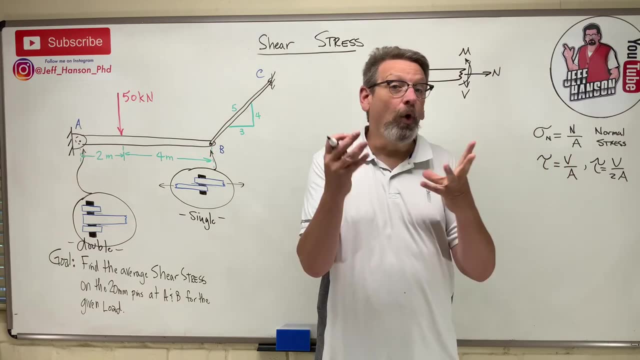 have to tell you something about the pin. so you know, are we talking single sheer or are we talking double sheer? So how do we find V the sheer pin? So we have to tell you something about your force on the pin. Well, you know what we have to do. You're not going to believe this. 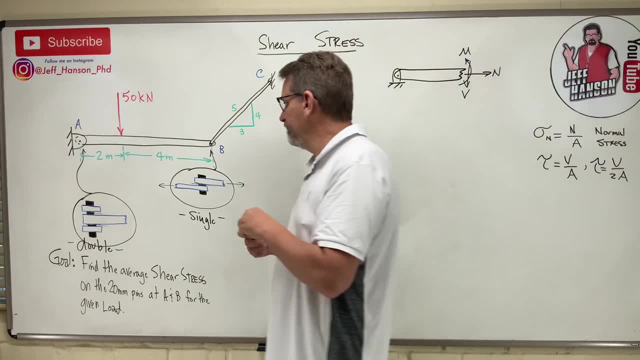 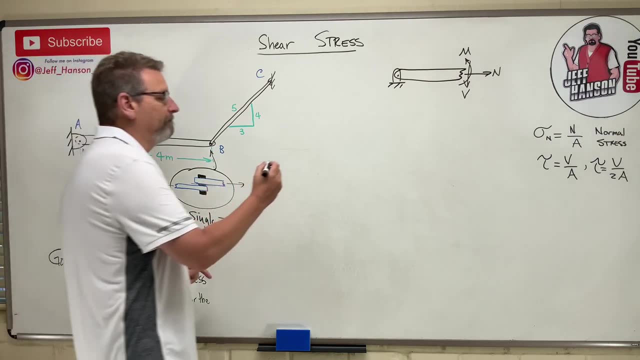 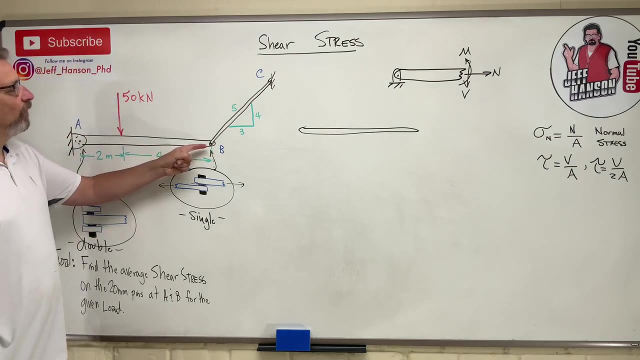 We're going to have to do some statics. What? Yes? And that would start with what? do we start every problem off with Free bike diagram. Let's draw this beam here. okay, Here's the beam. That's a great beam. What do you do? What does this guy over here, what does V see? 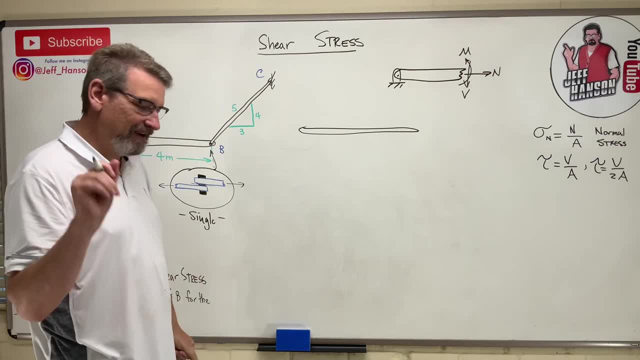 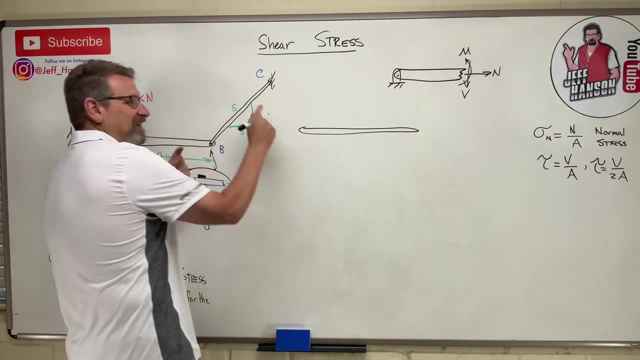 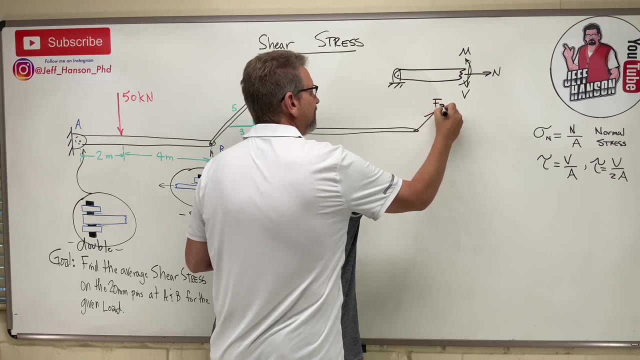 It's pin connected at both ends. no forces in the middle. That's a two force member. That's right. And as I pull down on this, I'm stretching that guy so he's in tension, so I can feel him pulling on me, right? So this is FBC, okay, And remember, FBC also has 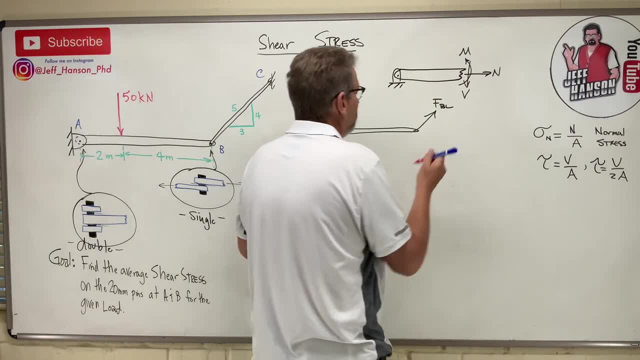 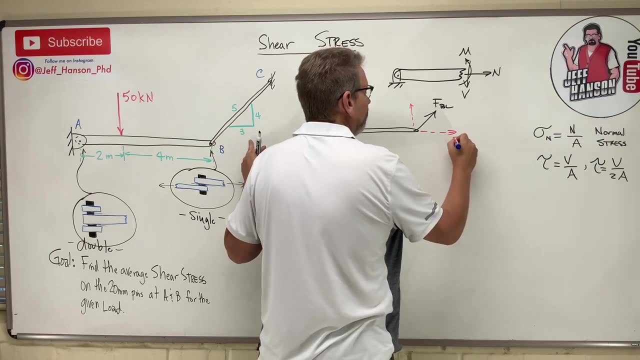 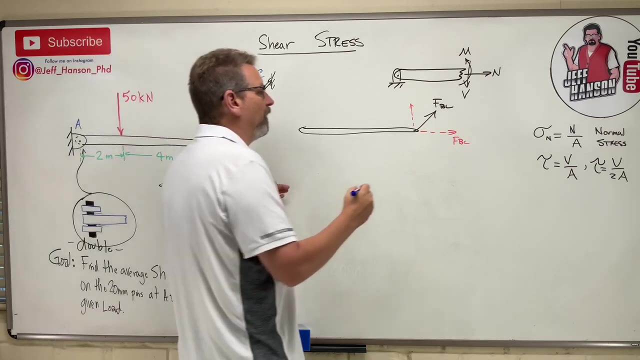 he's going to have two components, isn't he? And he's a three, four, five. So he's going to have one here and one there, And this one's going to be FBC, FBC times. how much Remember? the X uses the X side of the triangle, over the hypotenuse. So 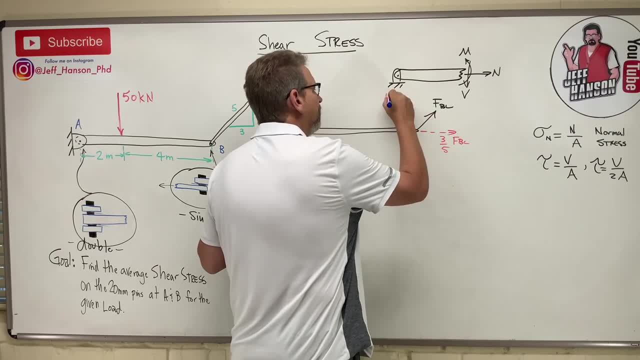 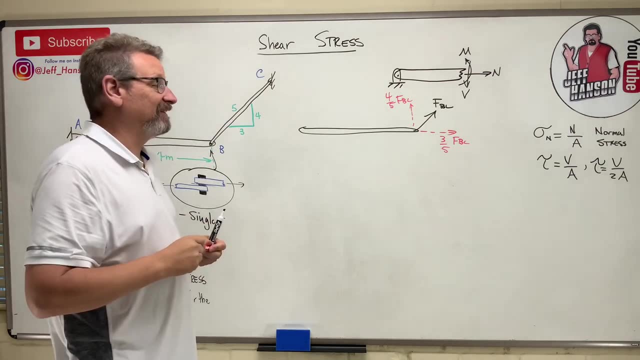 three-fifths, And this one up here, four-fifths- FBC. okay, Guys in solids, you're going to be expected to know this like automatically. You're not going to have to be like I have to go back. 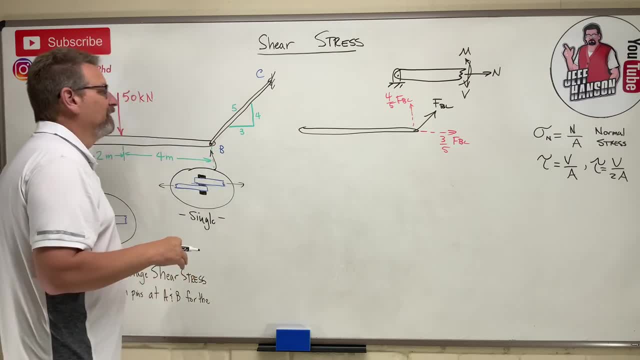 and review statics. You're going to be in trouble, okay, We got to just know, okay. And then what else that goes on our beam Over here. A is a pin connection. Now for statics. I don't care. 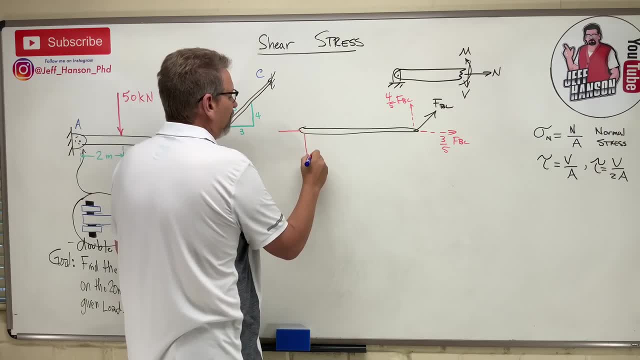 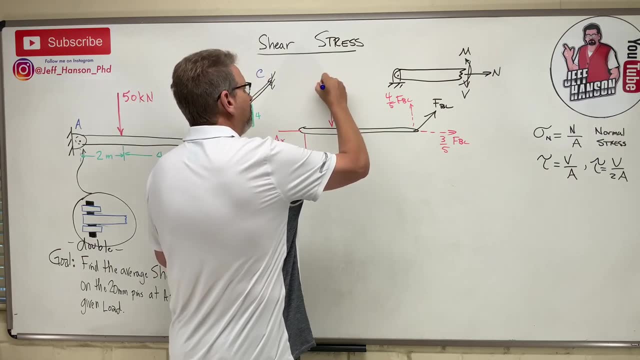 that it's a double or single. All I care about is a pin connection. So it's going to have an AY and an AX, And then over here is that 50 kilonewton load. okay, So which way does AX have? 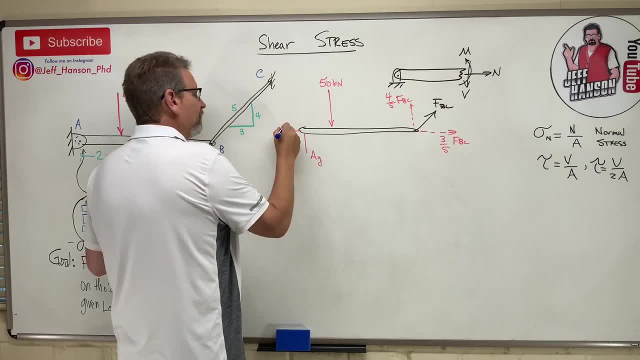 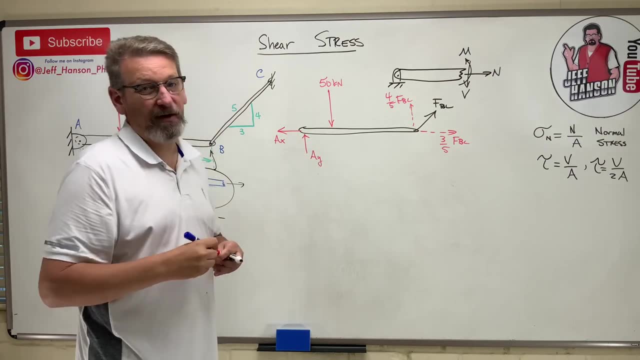 to go. Well, that one goes to the right, So this one needs to go to the left. And which way does AY have to go? I think probably up, And at this point I can still guess if I get it backwards. 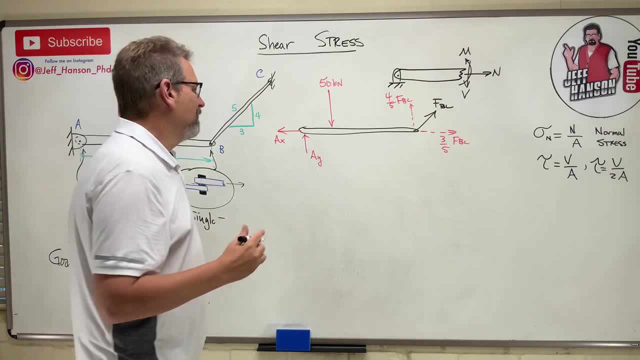 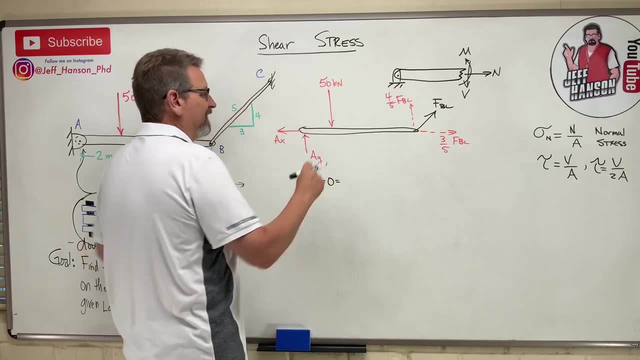 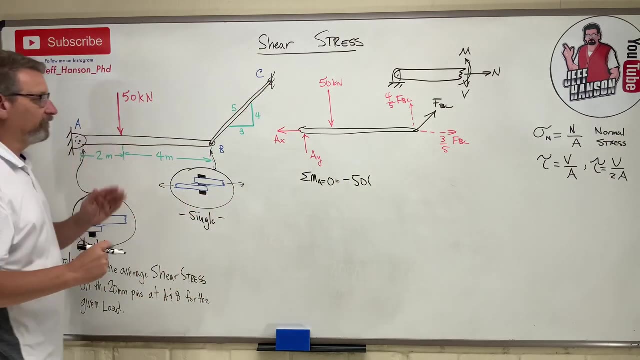 I'll just get a negative. But I don't think I'll get a negative right, Okay. so how about some of the moments at point A? And what do we get? We get the 50 rotating as negative. So minus 50 times, how far away from point A is that? Well, it's two, It's two, And then I get this guy's a. 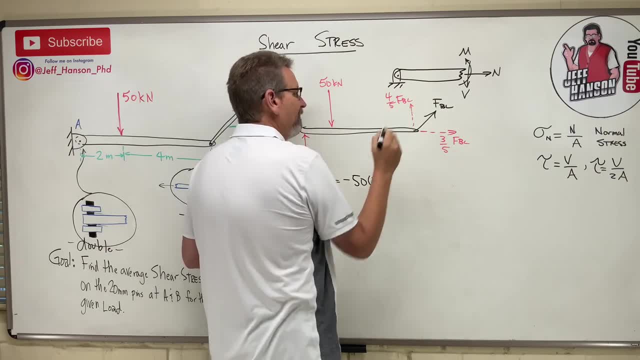 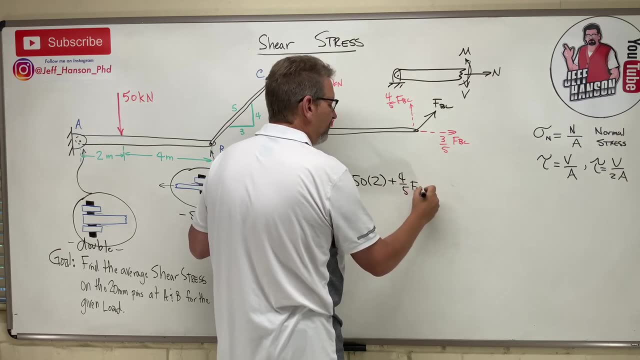 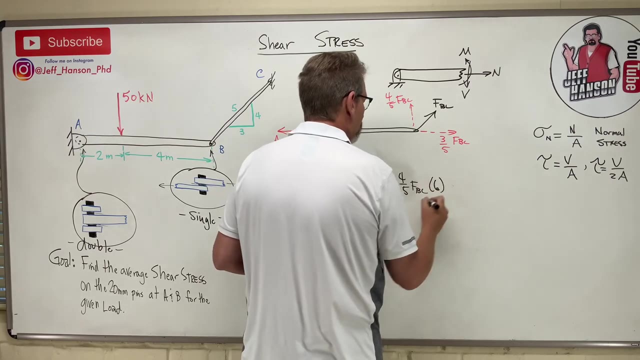 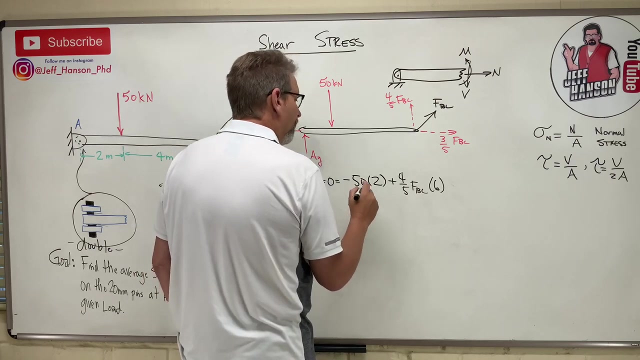 cha-cha force which, ah right, He goes through point A. Then I got that guy which rotates me positive plus four-fifths FBC times. how far away is that guy? Two plus four, how about six? Okay, All right calculator. So 100 times five divided by four. 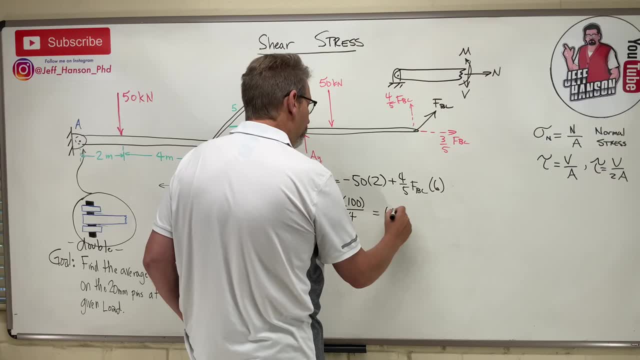 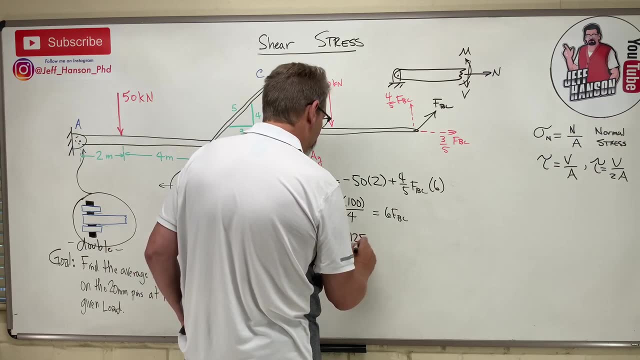 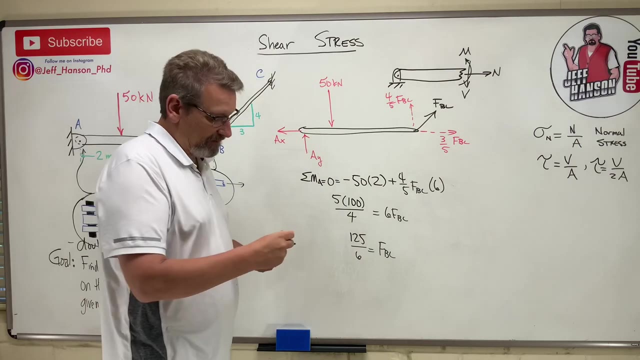 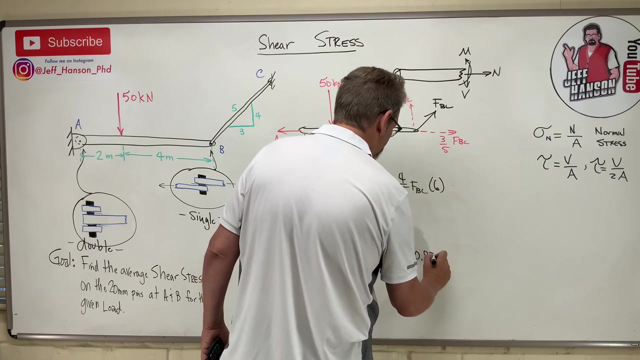 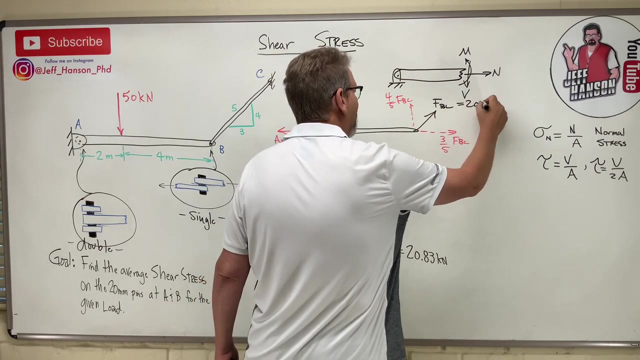 right equals six FBC. 500 divided by four is 250, 125.. So 125 over six equals FBC. And how much is that? All right, On 125 divided by six: 20.83.. So now I know that guy: FBC right, 20.83.. Okay, kilonewtons. 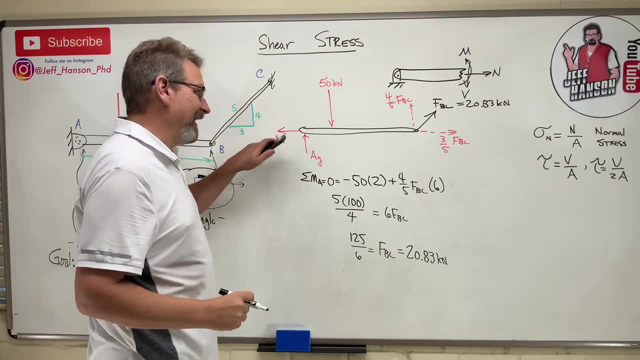 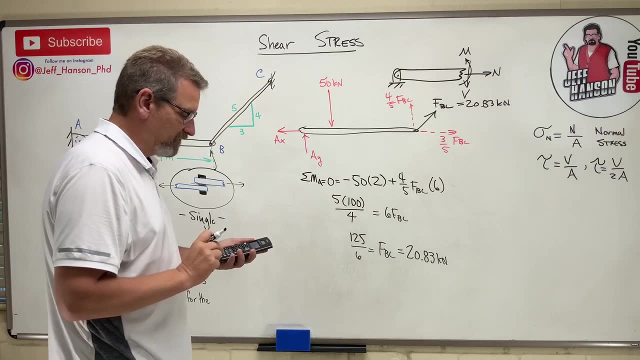 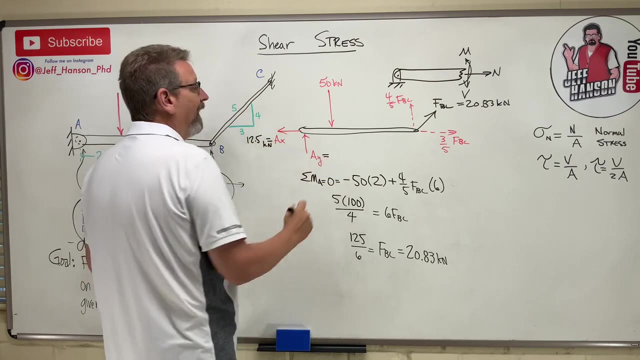 And how do I find AX? Well, AX is going to be equal to that guy right there, So that would be 20.83 times 0.6, which is 12.5 kilonewtons, And then AY. 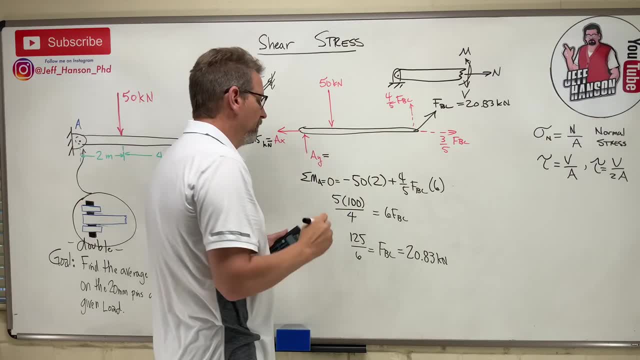 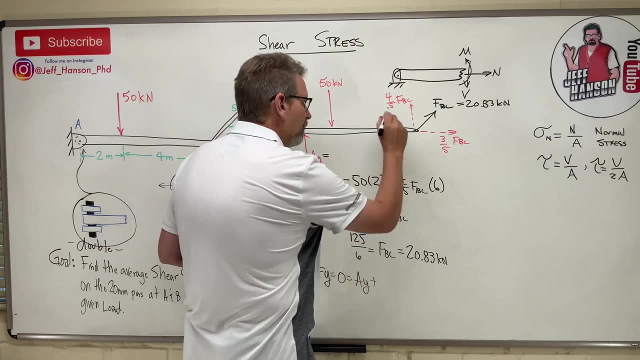 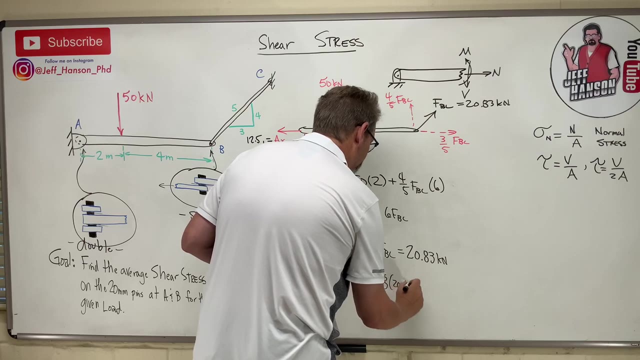 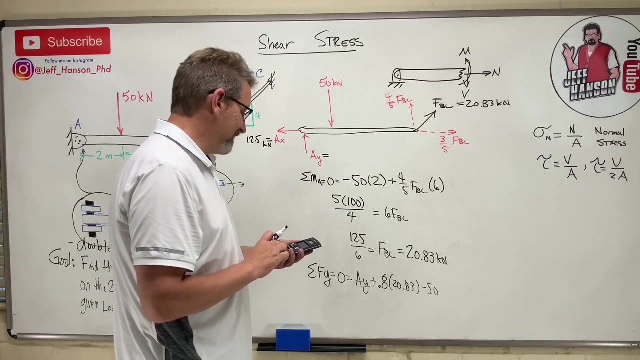 right, the two upstuffs have to equal the downstuff, right? So sum of the forces in the Y equals AY plus that guy, 0.5.. 0.8 times 20.83 minus 50.. And so AY equals what? 50 minus 0.8 times 20.83, 33.34.. 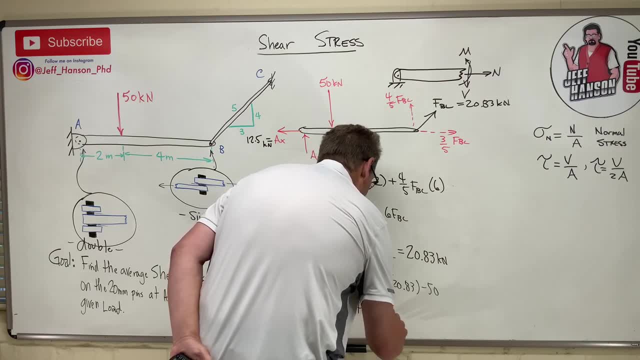 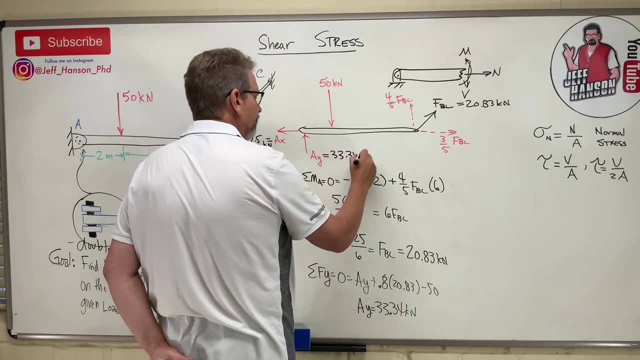 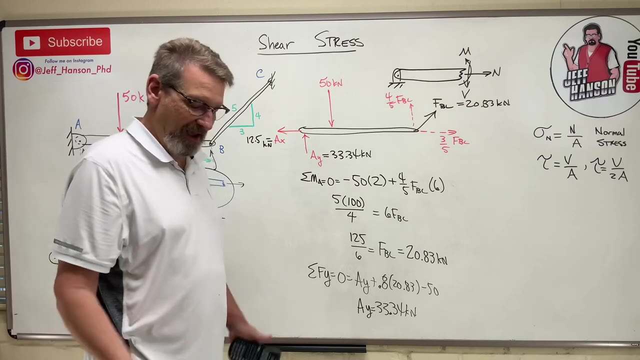 So AY kilonewtons, Okay. So that goes here. 33.34.. 34 kilonewtons, Okay. So you see how we got that. That was a statics problem, man. You see how important statics is. Come on y'all. Luckily you had the world's greatest statics teacher. 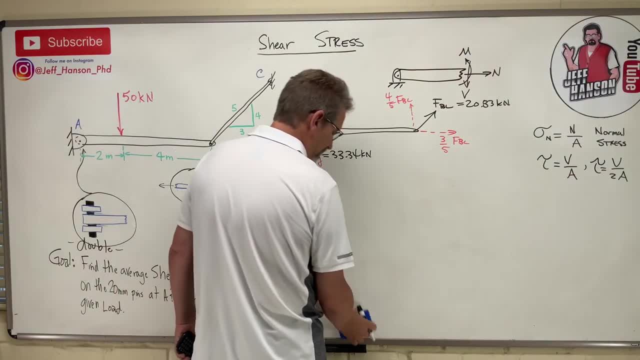 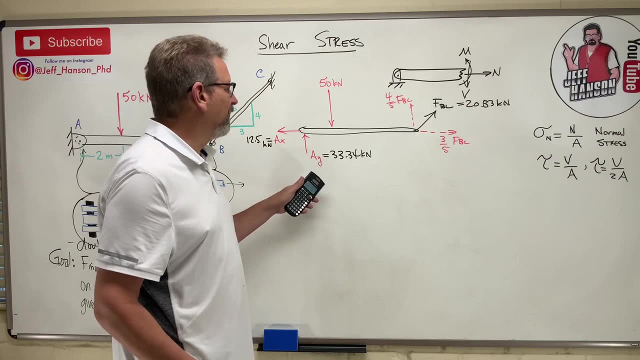 didn't you? Well, only if you followed my statics series, then you did. Okay, Let's see if we can do this now. Next, we got to do this, Okay, So we're going to have one case of single shear, one case of double shear, And then we're going to have one case of double shear. 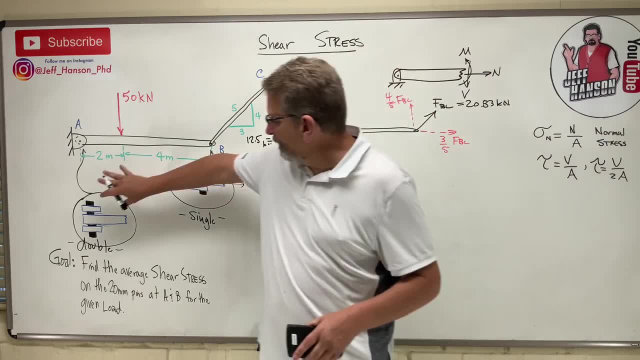 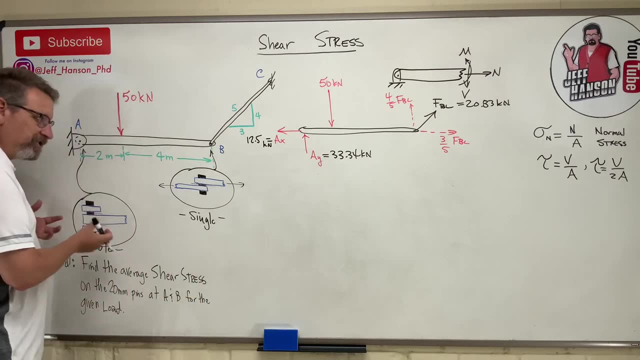 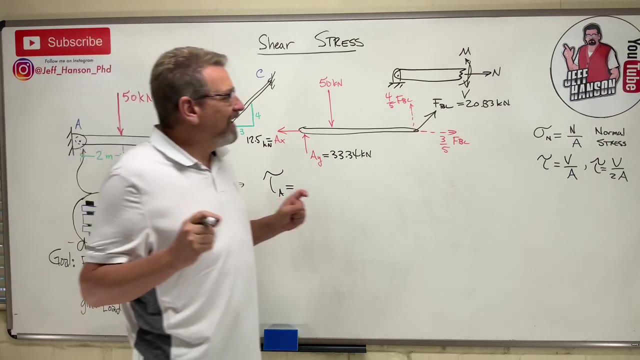 The single shear is at pin B and the double shear is at pin A. Okay, So, let's do pin A. Let's do pin A. That's the double shear. Okay, So tau at point A is equal to: okay. what is V? What is V? Well? 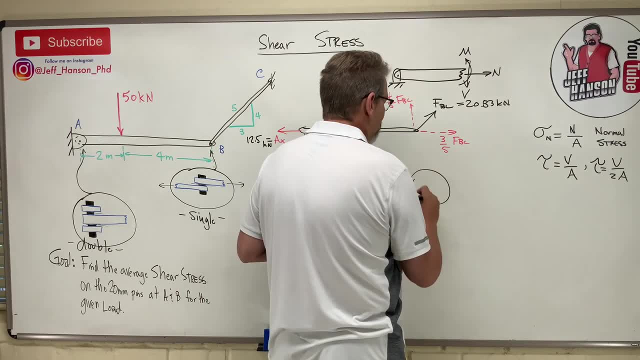 you know what? All of these are going to have the same A, aren't they? We have a 20 millimeter diameter pin. Okay, So A is equal to V. Okay, So we're going to have a 20 millimeter diameter pin. 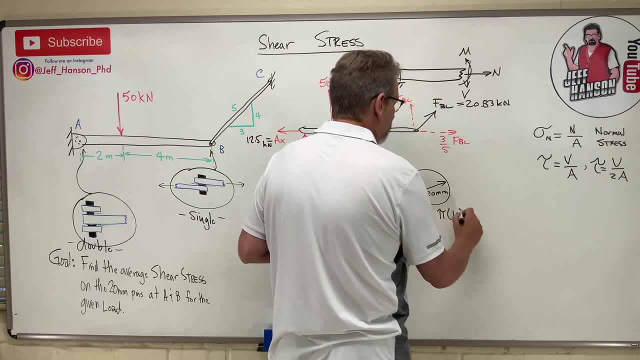 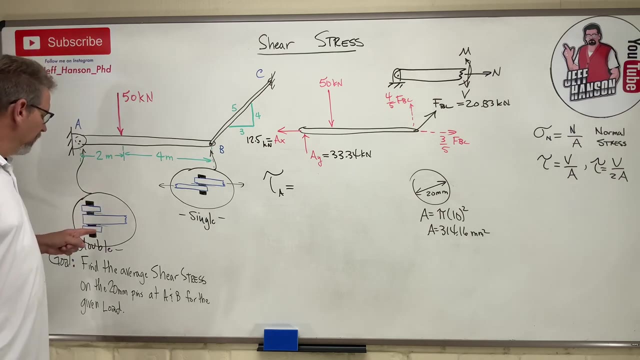 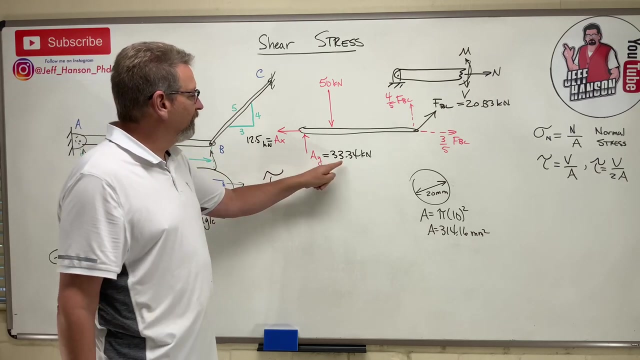 So tau at point A is equal to pi times 10 squared, which is equal to 314.16 millimeter squared. Okay, So here we go. The force at point A. what's the force on the pin at A? Well, you got 12.5 in the X and you got 33.34 in the Y. So how do you find the, the, the result of that? 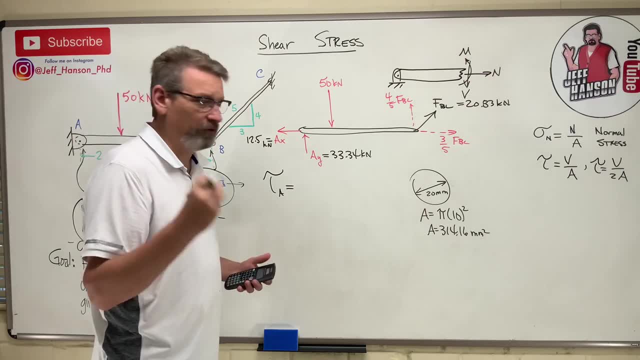 Okay, So tau at point A is equal to pi times 10 squared, which is equal to 314.16 millimeter squared On A. the total effect of those two forces squared squared take square root right. So here we go. 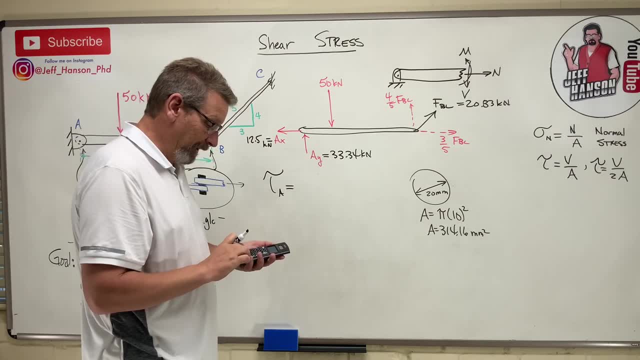 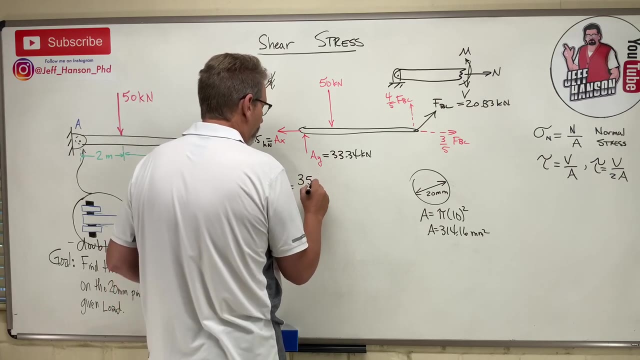 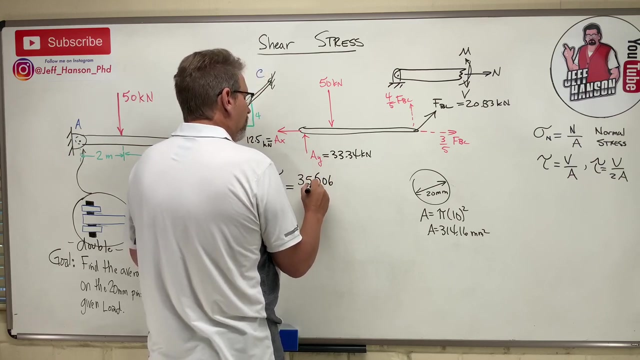 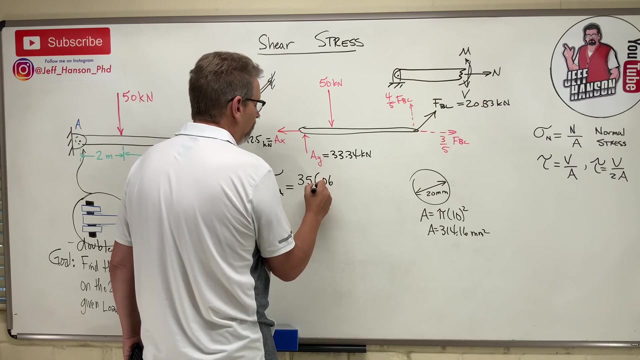 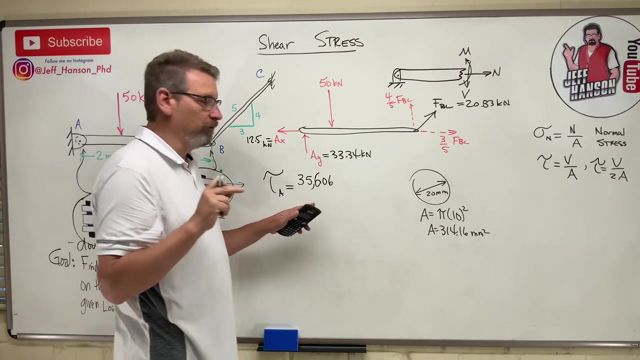 12.5 squared plus 33.34 squared equals inverse square root answer equals 35.6.. okay, well, wait a minute. how come you said 35.6 but you wrote 35,606, because this was given in kilonewtons. okay, so I just found that in kilonewtons and then I just 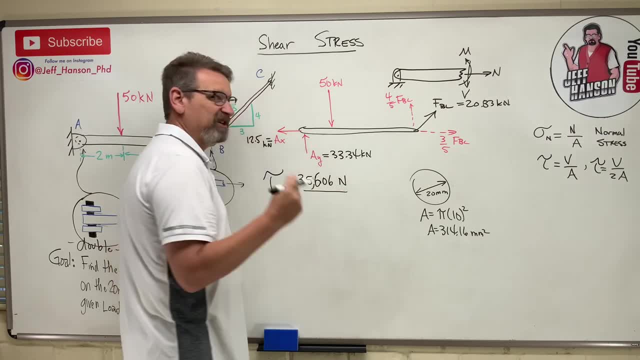 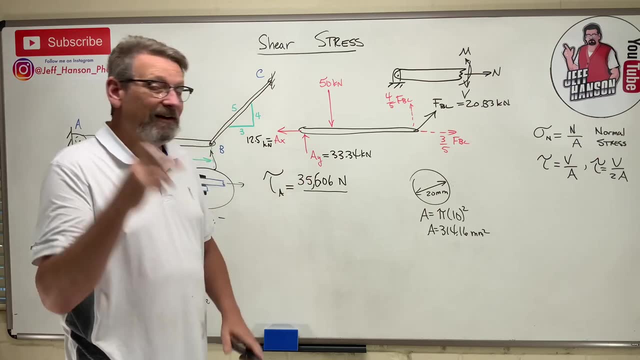 turned it into newtons. right, because kilos times 10 to the 3. so I just move the decimal over 1,, 2,, 3 places and I get this right. clever, because what is my area going to be? it's going to be 2. 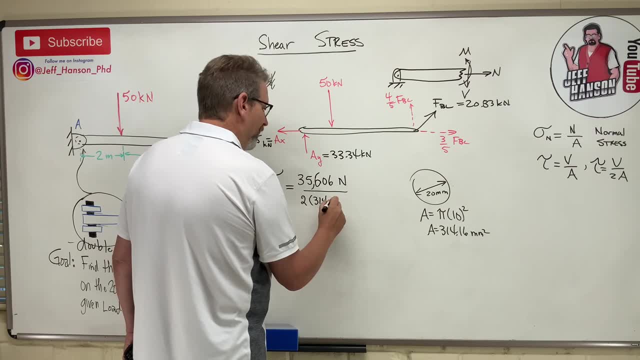 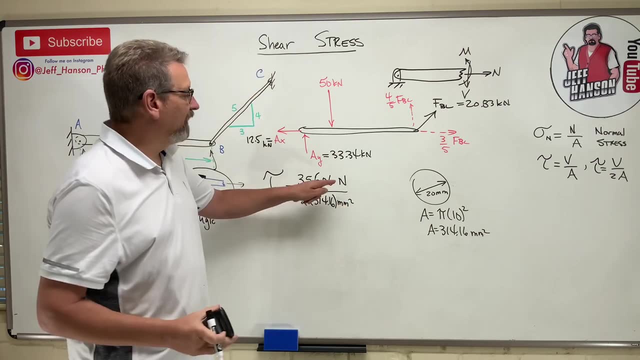 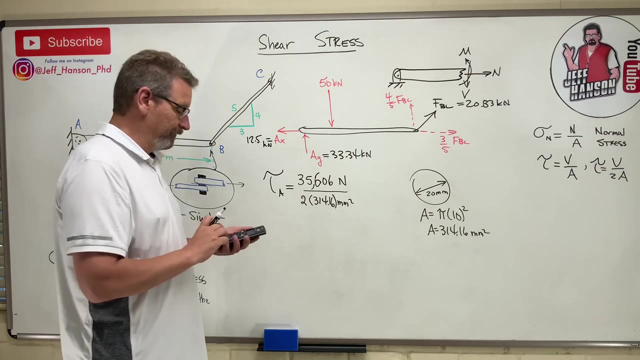 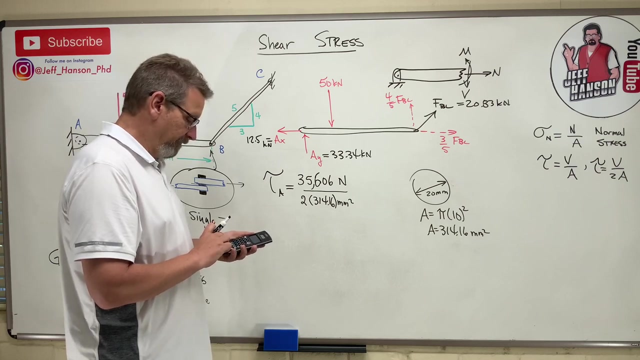 times 314.6, or 1, 6 millimeters squared. okay, and now, what is newtons over millimeters squared? that makes sense to me, right? so that's, that's megapascals, isn't it? so here we go: 35,606 divided by 2 divided by 314.16 equals 56.67. 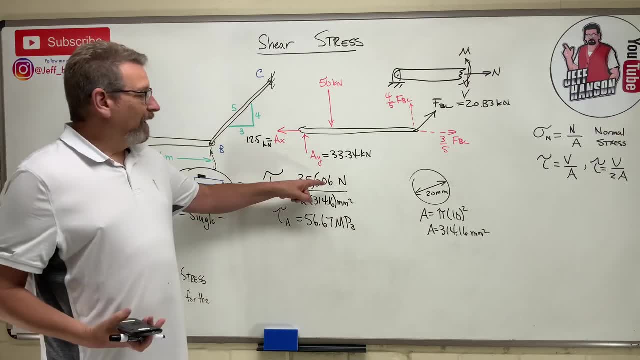 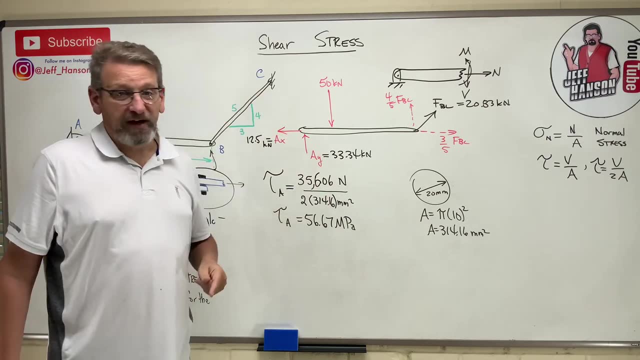 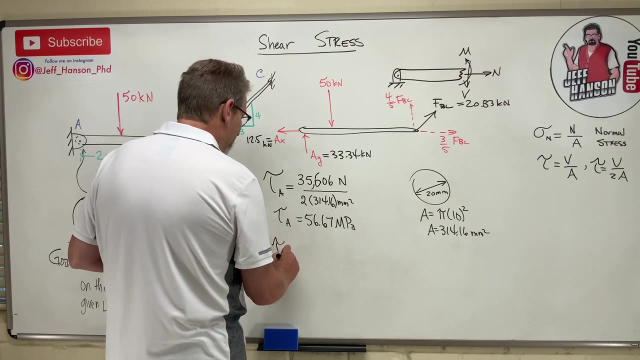 okay, I'll do this a bunch. I'll get everything in newtons and meters or newtons and millimeters. so in my mind I know, oh, that's a megapascal. okay, all right. so the next one's going to be what? tau for point b, and you'll notice the two there for the double shear. right now we're doing the single. 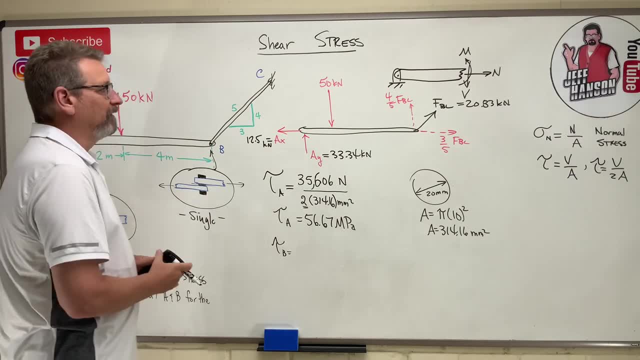 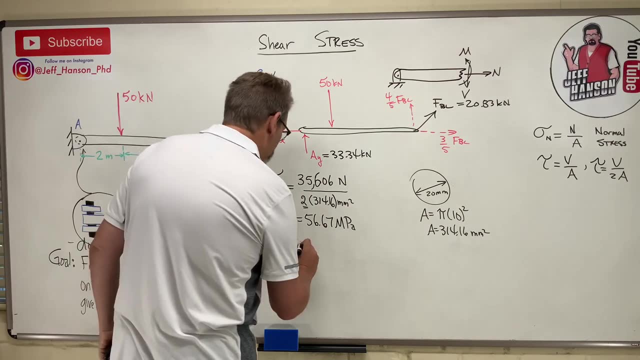 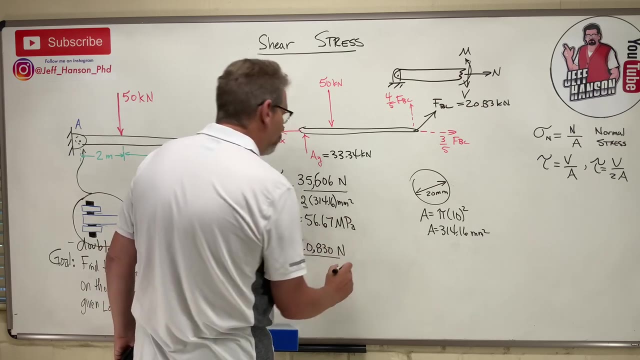 shear case. what's the force on this pin? well, the force on that pin is completely. there's just one force on it, it's 20.83. okay, so 20. oh, I'm going to do this- 830 newtons, because 20.83 was kilonewtons.